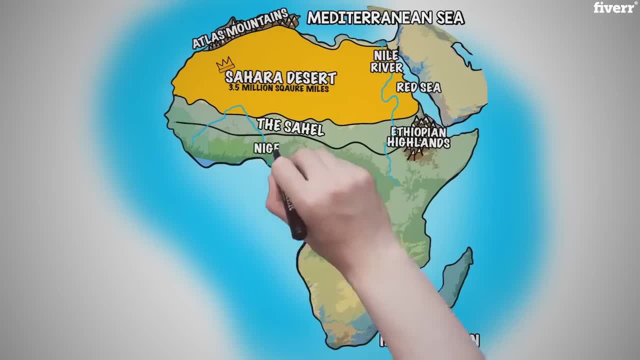 In West Africa. the Niger River originates in the Guinea Highlands in modern southeastern Guinea. It runs in a crescent through modern Mali, Niger on the border with Benin, and then through Nigeria, ending in the massive Niger Delta into the Gulf of Guinea in the Atlantic Ocean. 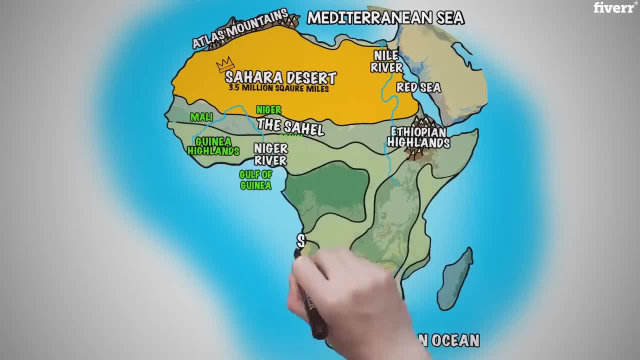 The lush savanna grassland makes up most of Africa and completely surrounds the rainforest of the Congo Basin in Central Africa, as well as the Niger River to the west and Lake Victoria, which sits south of the Nile River. The Kalahari Desert covers the southernmost tip of Africa and is the sixth largest desert in the world. 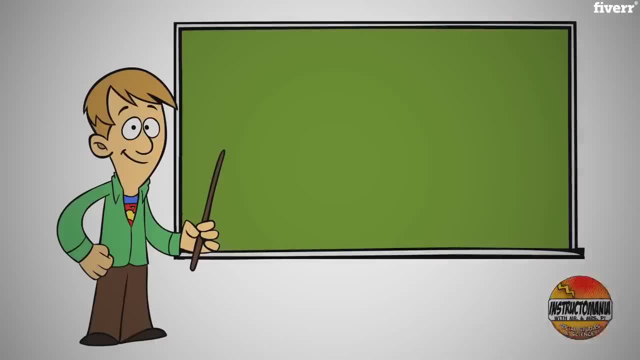 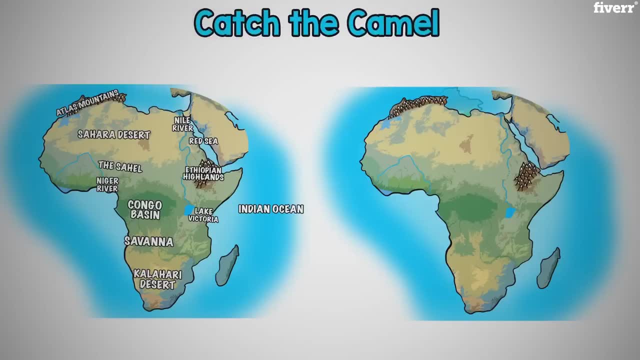 It has a radius of 4.1 km and the radius of Tamik. Testing your knowledge, Let's play Catch the Camel. In this game, you will track the camel as it appears on a blank map of Africa. Once the music stops, you will use an Africa map labeled with physical features to determine where the camel ended up. 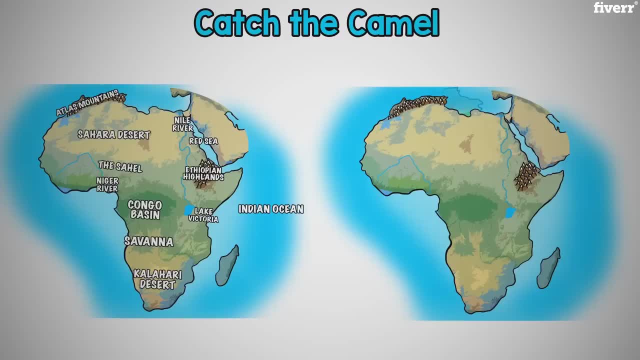 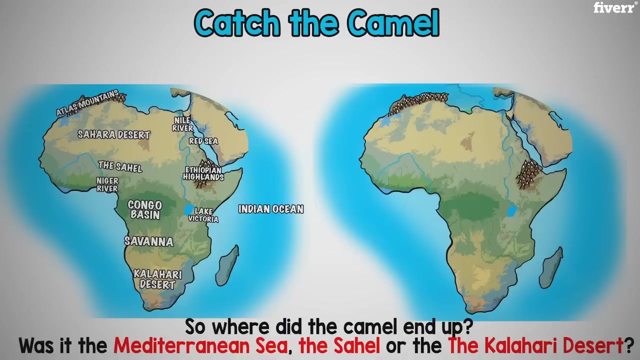 Other animals may appear on the map, so don't forget to keep your eyes on the camel. So where did the camel end up? Was it the Mediterranean Sea, the Sahel or the Kalahari Desert? That's right, It was the Kalahari Desert. 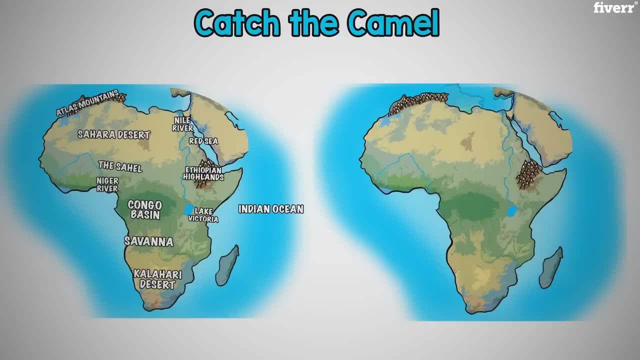 Let's try it again Again. remember to keep your eyes on the camel. So where did the camel end up? Was it the Savannah, the Niger River or the Red Sea? It was the Niger River. Let's try one last time. You got this. 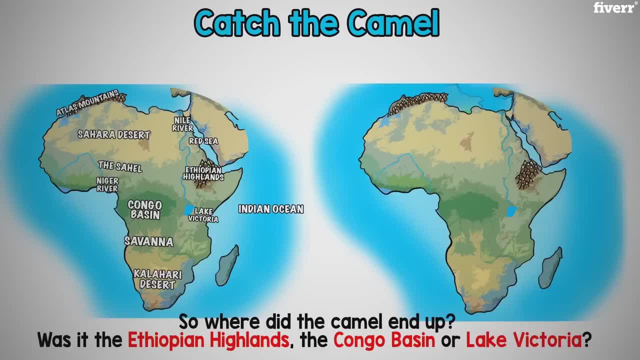 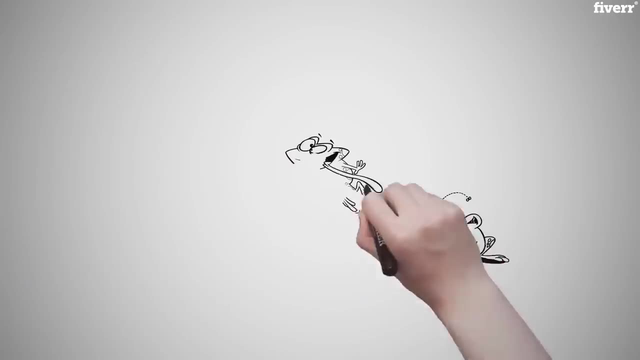 So where did the camel end up? Was it the Ethiopian Highlands, the Congo Basin or Lake Victoria? Nice job, It was the Ethiopian Highlands. It was the Ethiopian Highlands. Here's a freaky fact: The largest frog species in the world, the Goliath frog, lives in West African lakes and rivers. 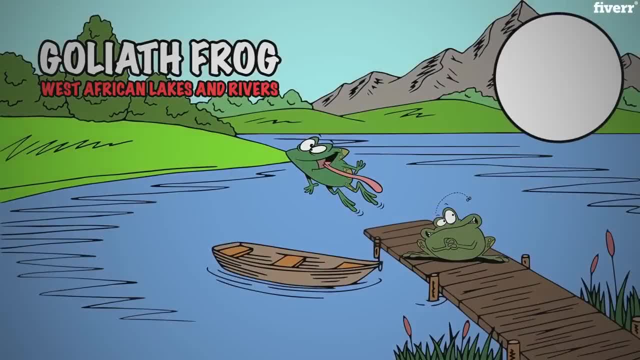 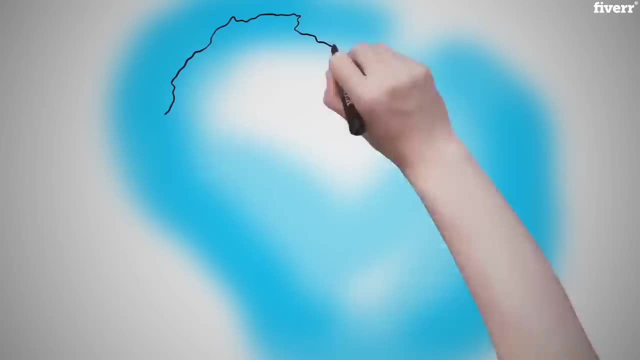 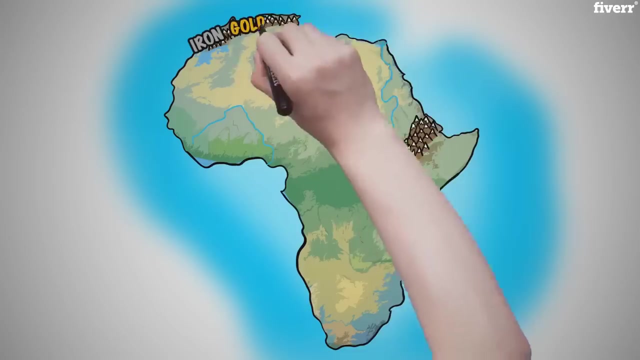 They grow up to a foot long and weigh up to eight pounds. Goliath frogs are nearing extinction because they've been a food source for humans. Section 2. How Geography Shaped the Lives of Medieval Africans. Natural Resources- Natural Resources Found in the Atlas Mountains and Ethiopian Highlands, such as iron, gold and salt, offered wealth to the inhabitants. 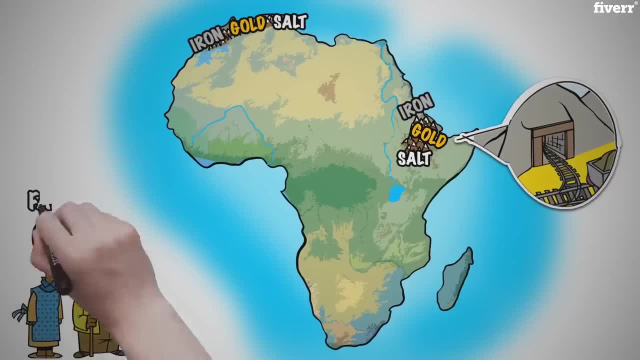 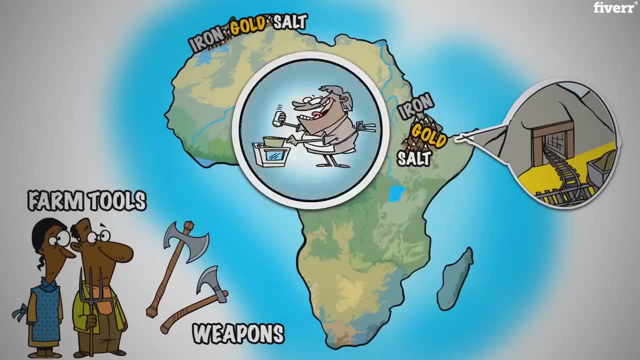 Africans traced back to the Nok culture and later the people of medieval Ghana crafted iron into farm tools and weapons for defense. Salt mined in northern Africa aided in preserving and flavoring food. Eventually, regions were conquered for these resources. Trans-Saharan trade routes crisscrossed North Africa. 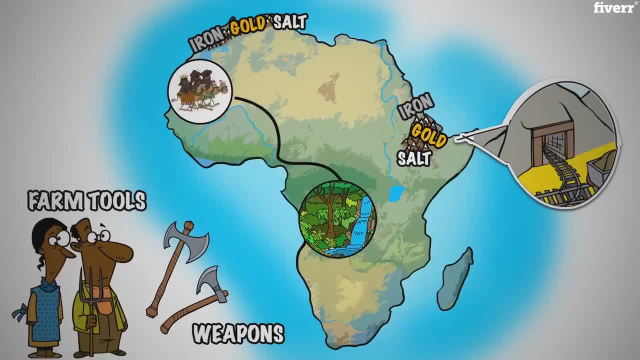 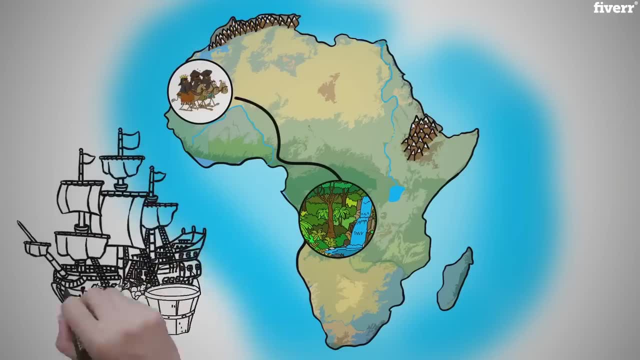 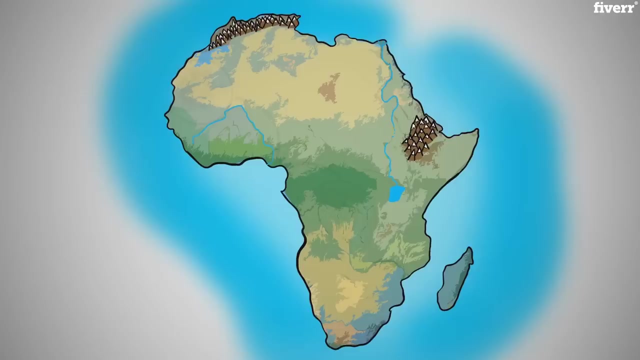 North Africa, from the Sahara Desert to the gold-rich rainforest region of South-Central Africa. The Niger River offered water, food and transportation to Western Africa, especially for the medieval African trade kingdoms of Ghana, Mali and Songhai. The rich soil along its banks allowed for farming and its plentiful water allowed for crop irrigation. 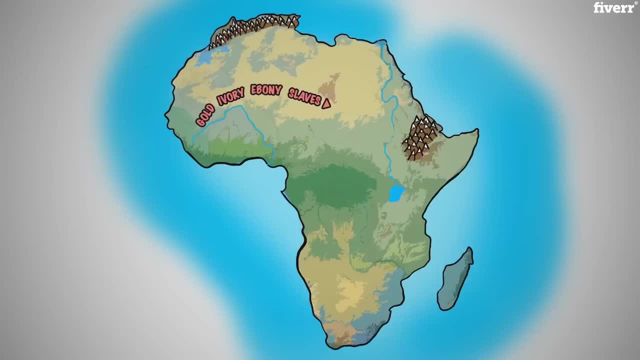 Gold, ivory, ebony and slaves from West African kingdoms were also used for farming. Gold, ivory, ebony and slaves from West African kingdoms such as Ghana, Mali and Songhai were sold in North Africa and the Middle East. They were traded for salt and copper mined in the Sahara. 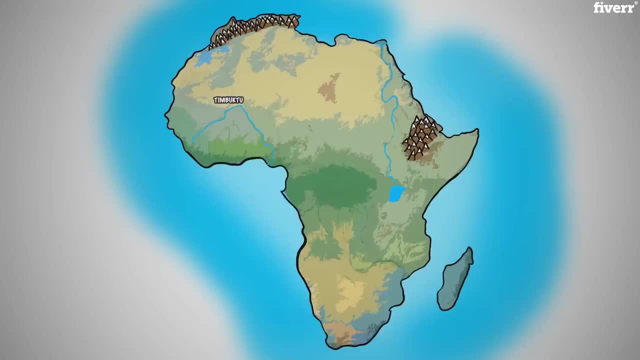 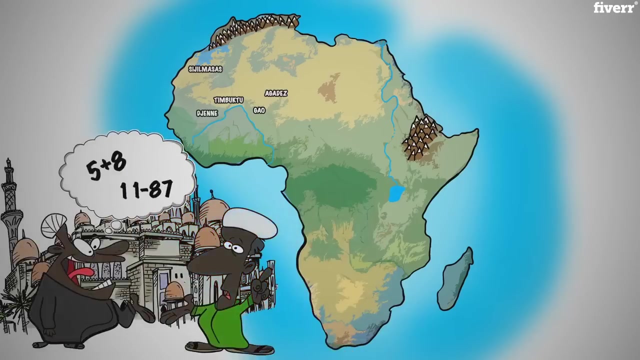 In Western Africa, the major trade centers were cities such as Timbuktu, Gao, Agadez, Sijilmasa and Djenne. A thriving gold-salt trade eventually led to the exchange of ideas. Islam made its way to Africa as well as the advanced knowledge of the world. 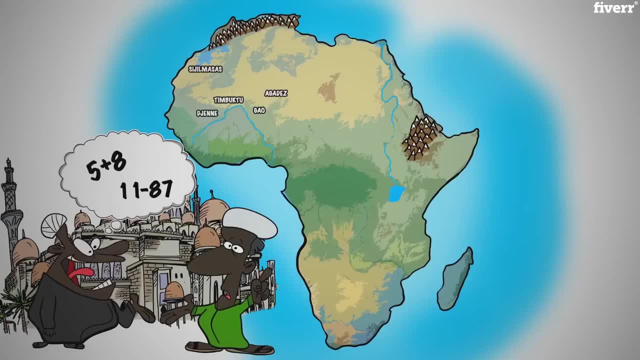 Islam made its way to Africa, as well as the advanced knowledge of science and math from Muslims, Indians and Berbers. The medieval African kingdoms of Ghana, Mali and later Songhai grew to cover most of West Africa, seeing many cycles of conquest paired with economic and cultural success. 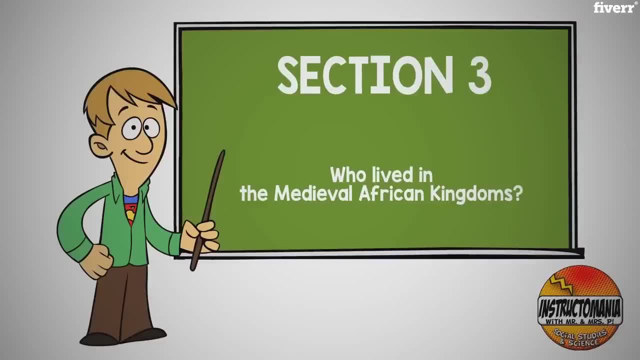 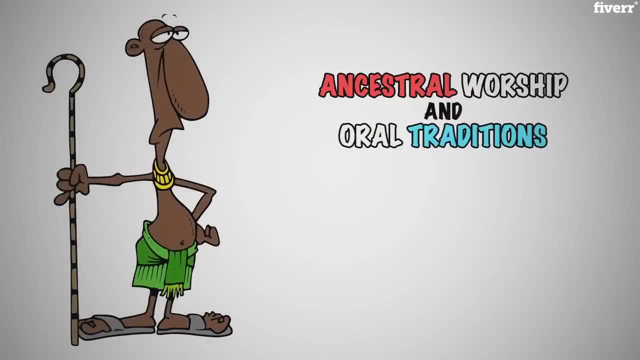 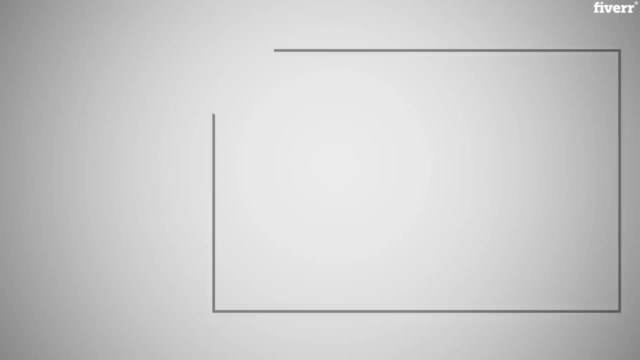 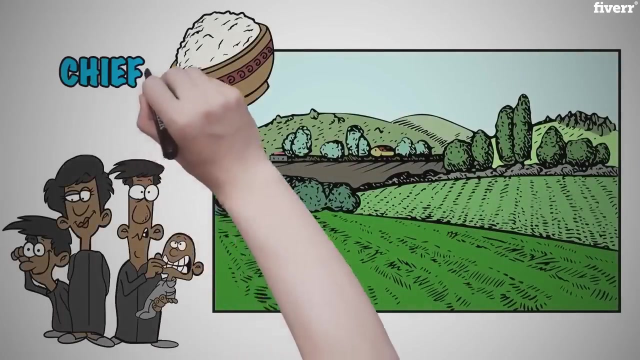 Section 3. Who Lived in the Medieval African Kingdoms? Africa's early tribes believed in ancestral worship and oral traditions. The griot of each village maintained their history and legends and was highly respected. Village farmers grew rice and millet. Family villages greatly relied upon an extended family. 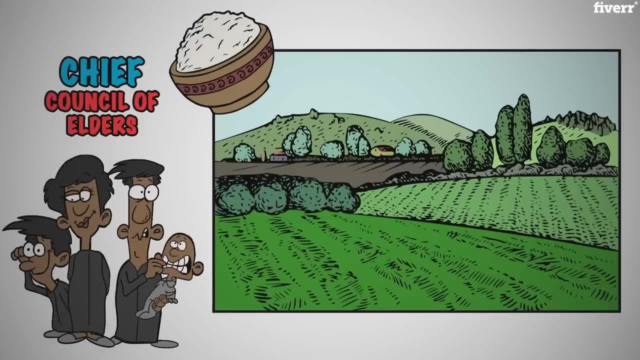 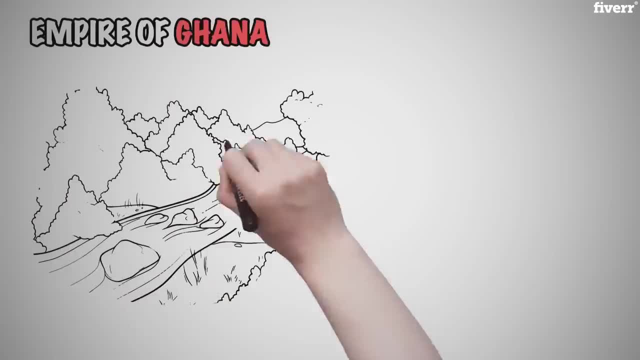 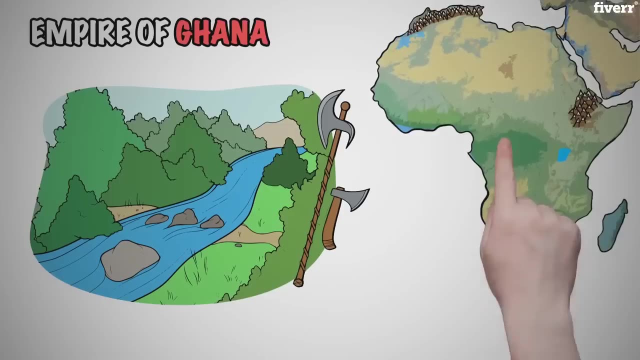 which included a chief and a council of elders to govern, divide farming responsibilities and maintain order. Eventually, the Empire of Ghana rose next to the Niger River, using iron tools to farm and to conquer neighborhoods. The之 vorher قرنواенные آراماً. 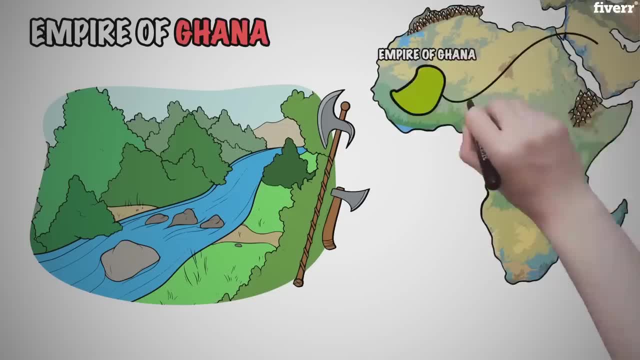 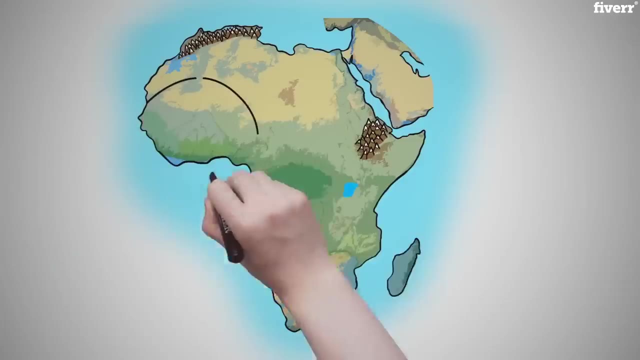 Later, Muslim traders called Almoravids traversed from the Arabian Peninsula and attempted to take over the Kingdom of Ghana. The Muslims failed to conquer it, but weakened it enough that rebellion and war between African tribes became common. Eventually, Ghana was conquered by Mali, which grew to be roughly twice its size. 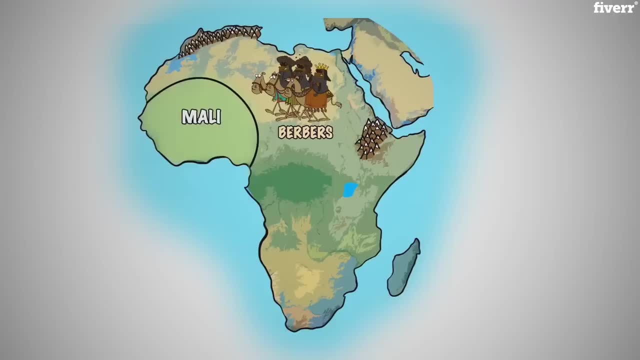 Caravan traders called Berbers originally crossed the Sahara Desert. Caravan traders called Berbers originally crossed the Sahara Desert to trade for food and water. trade with the African kingdoms such as Mali and the rest of the medieval world Sea trade with Europe and Asia also brought prosperity to the African kingdoms. 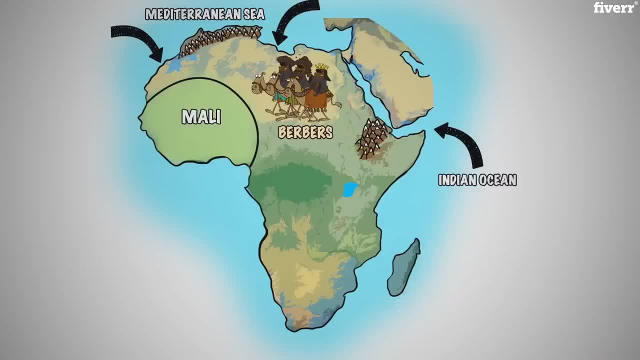 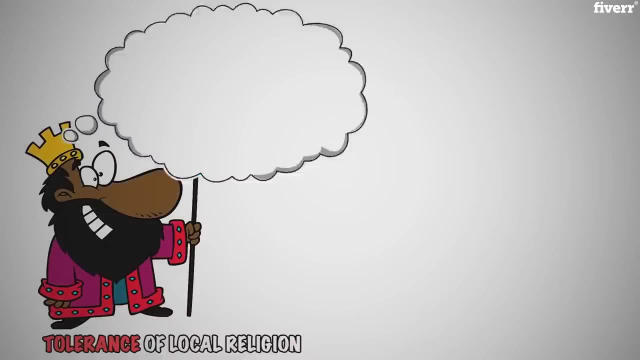 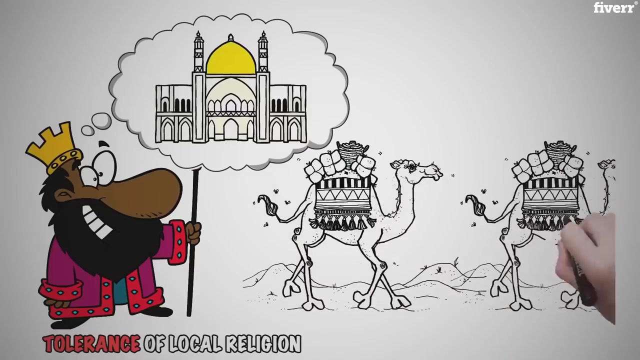 via the Mediterranean Sea and the Indian Ocean. The most noted leader of the kingdom of Mali was the Muslim Mansa Musa. He practiced tolerance of local religion, even though he had converted them to Islam When he traveled to Mecca for a religious pilgrimage. 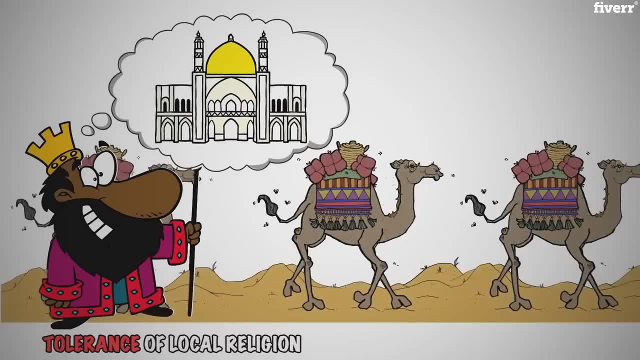 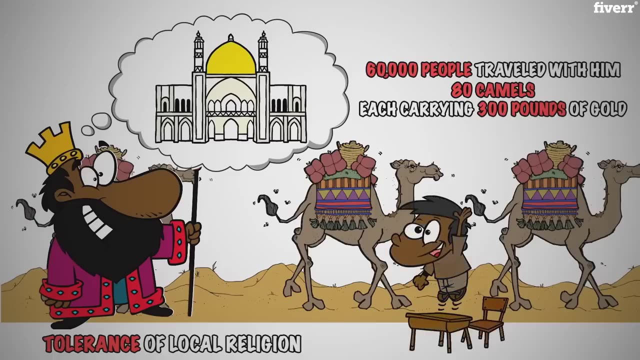 he brought an impressive caravan that revealed the wealth of his people. Over 60,000 people traveled with him and 80 camels each carrying 300 pounds of gold. He welcomed Muslim scholars to be a part of his empire and study there. 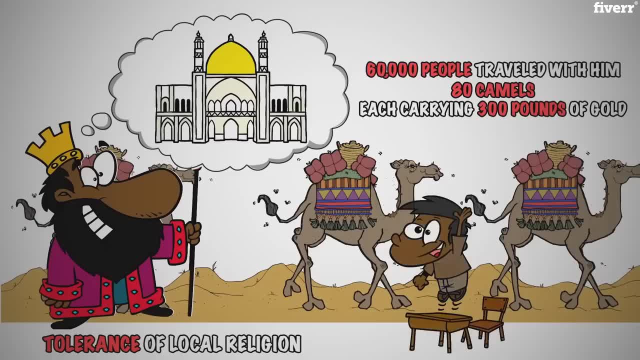 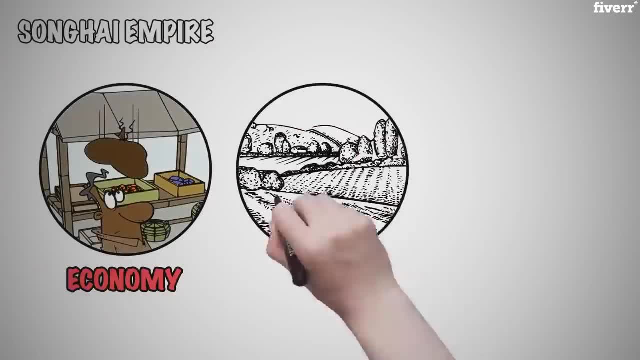 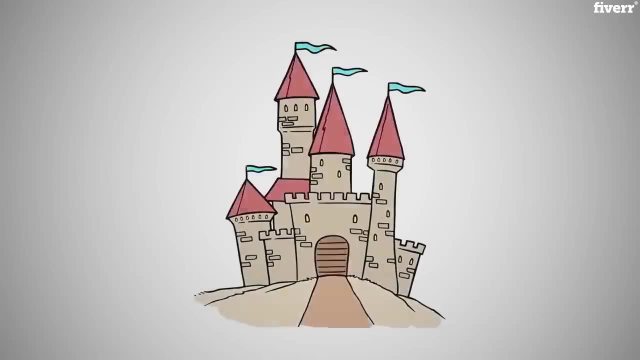 Timbuktu became a center of learning. under his reign, The last of the three major African kingdoms, Songhai continued to develop the economy, agriculture and scholar achievements of northwestern Africa. However, Moroccan troops captured salt and gold mines and broke Songhai into dozens of military camps.